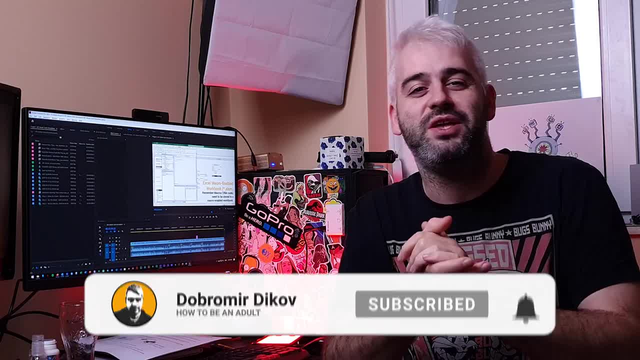 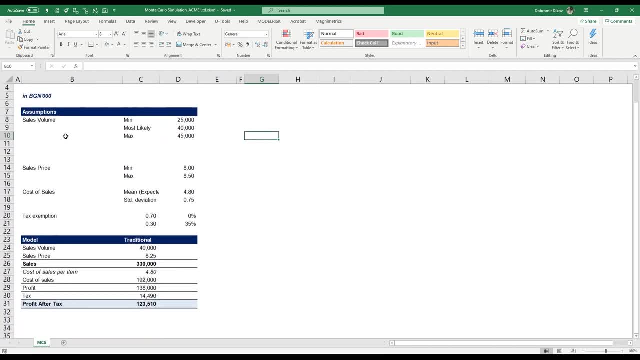 sub and maybe even a thumbs up. if you enjoyed the video, Let's get straight to it. Okay, so we have here this simple model where we have our sales volume, sales price, cost of sales and our option for tax exemption, and I've went ahead. 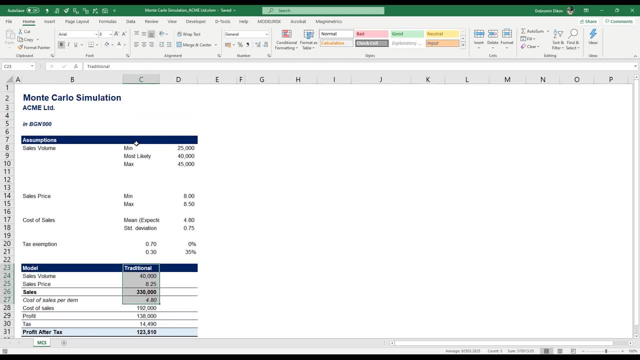 and calculated the traditional approach. So let's look at what we have done. Our sales volume is so. it's gonna be minimum 25,000, most likely about 40,000, maximum 45,000 and for our traditional model we would have gotten: 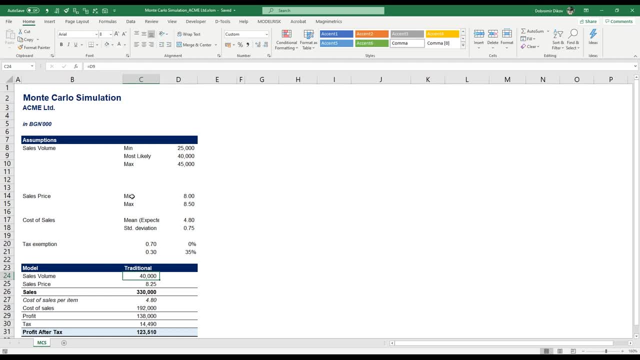 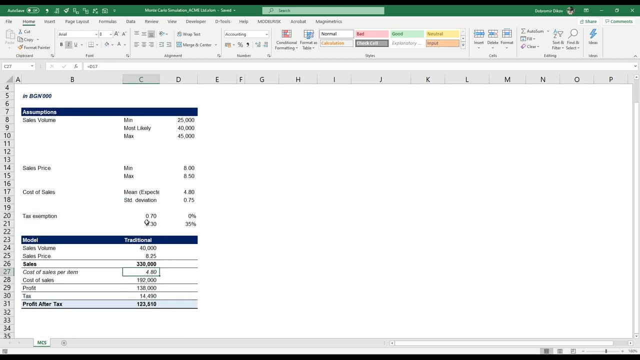 the most likely. Then our sales price. we have a min and a max, so I just went ahead and calculated an average and for our cost of sales we have our mean, which is the expected and our standard deviation taken that expected here. And for our tax exemption, there's 70% chance that we're going to get 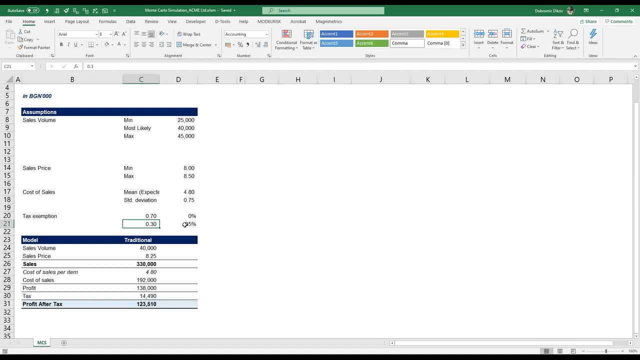 the tax exemption and 30% chance that we're not going to get exempt. So we're going to have to pay 35% tax And we use a decision tree formula here. So basically we get the probability multiplied by the outcome plus the other probability multiplied by that outcome. 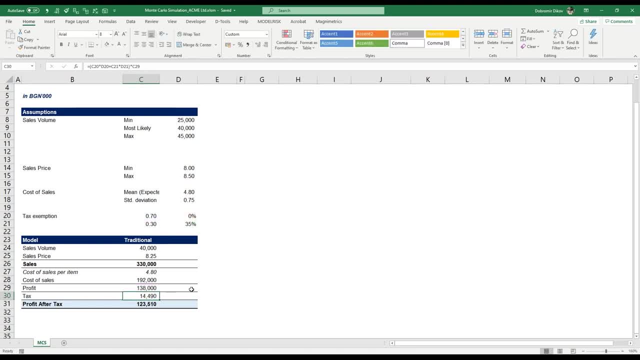 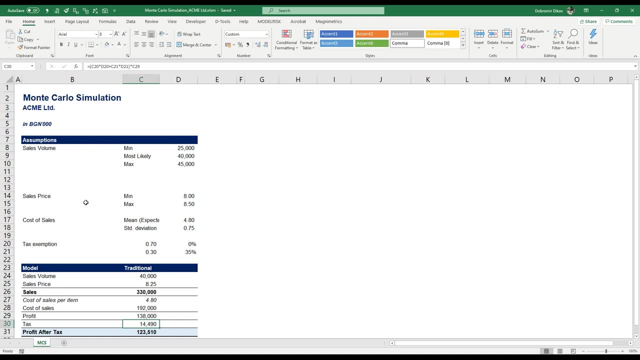 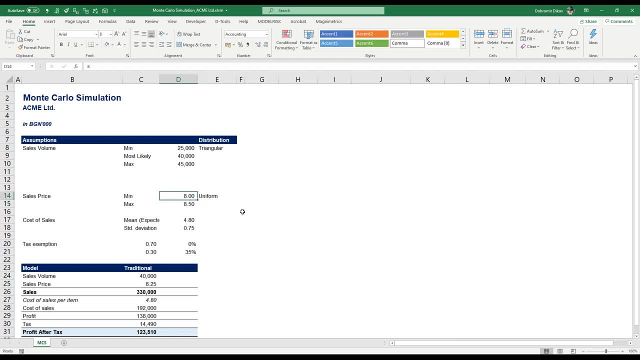 Okay, so this is a triangular distribution. we have a min, a most likely and a max. Okay, so this is a triangular distribution. we have a min, a most likely and a max. This here is uniform distribution, so min and max and everything is exactly the. 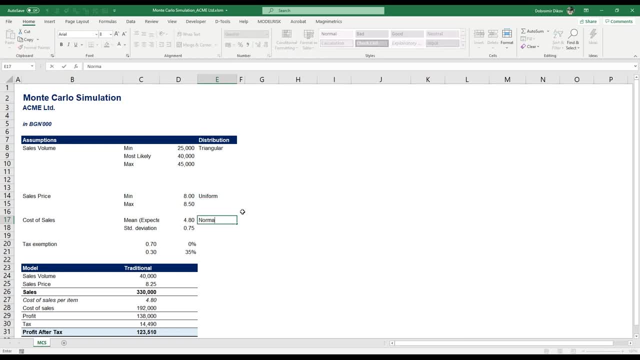 same probability of occurring. This is a normal distribution and this is a discrete distribution. We have a list of options, so it can either be this or this with those probabilities, and it can never be like 25 or something like that. Let's go ahead and calculate some values for those before we build our Monte. 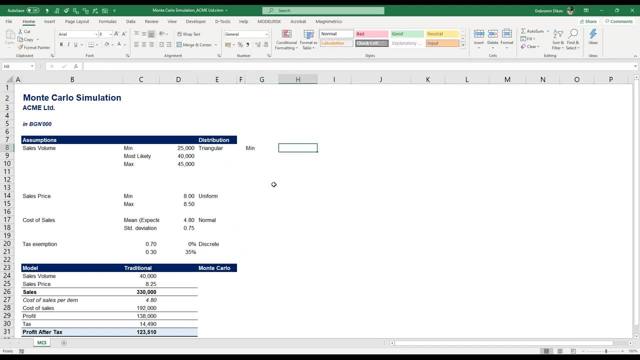 Carlo simulation. Here we'll need to set our min, our most likely and our max- and I'm gonna add some borders to those- or min, just link it from here: most likely and our max. and then for triangular distribution there's no formula in Excel, so we have to calculate it on our own. We have a. 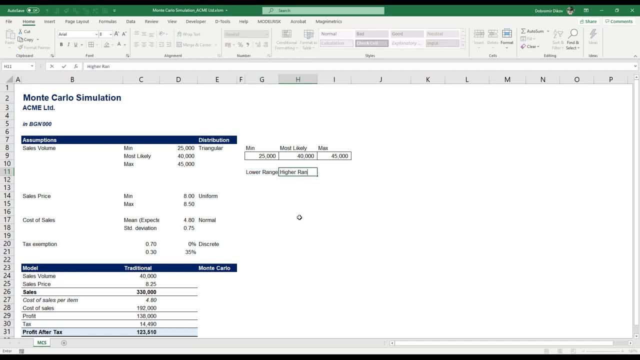 lower range, higher range. we have our total range and our cumulative probability, which is actually our random. Let's just format those as well. Our lower range is gonna be. Let me just carry over here some formulas for the triangular distribution, because it's a bit harder. 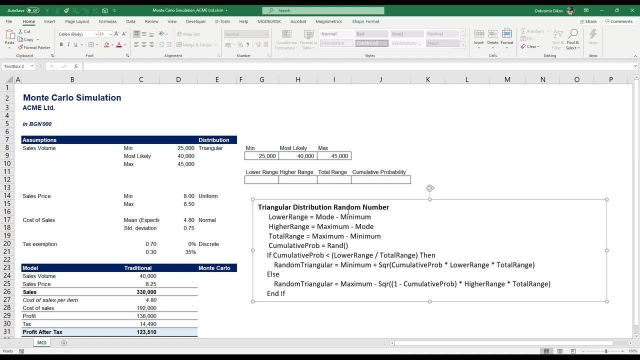 to to do So. here we have our triangular distribution, random number generation. So our lower range is our MOST, or most likely, minus our minimum. our higher range is our MAXIMUM minus our MOST. LIKELY, our total total range is our maximum minus our minimum, And our cumulative probability is just going to be the 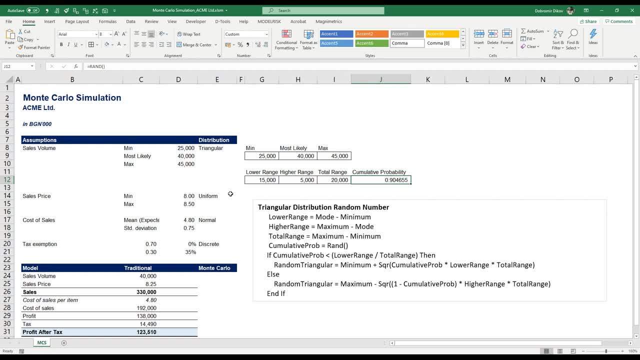 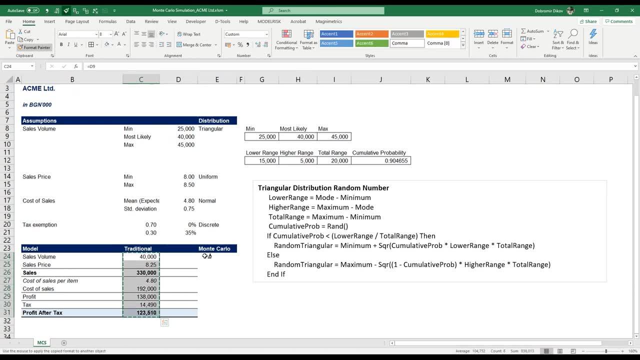 random number between zero and one. let's just go ahead and calculate it here for our model. there's going to carry all the formatting from here with the format painter And this formula. I'm going to carry over my profit, I'm going to carry over my cost of sales. I'm going to carry 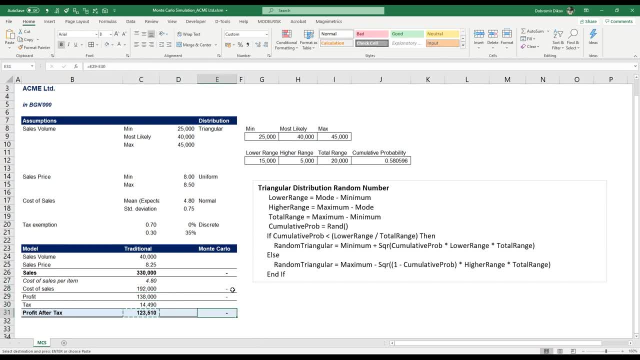 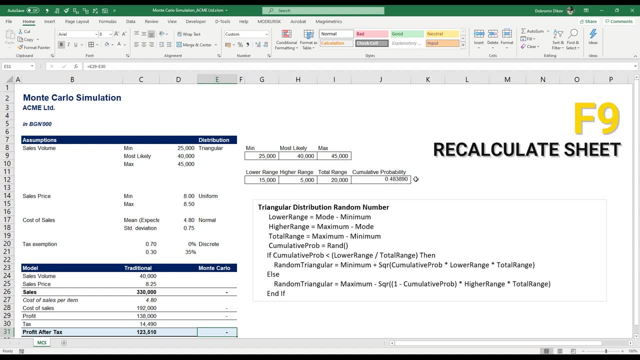 over and my net profit I'm going to carry over. you notice that every time we save or edit a cell or press f9, we recalculate the random numbers And this is what we're going to use for our Monte Carlo simulation. we're going to run it over and over and every time all the random probabilities. 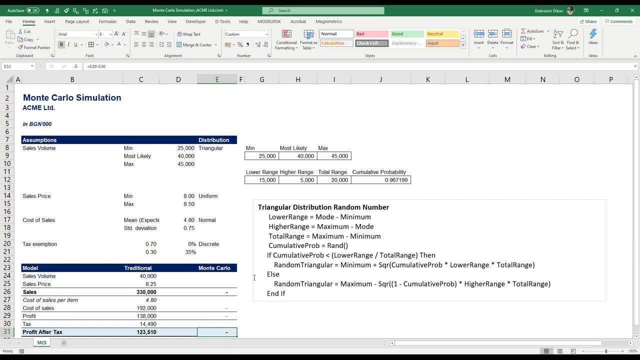 are gonna recalculate and we're gonna get a different result here. This is the formula that we have to write. It's a bit hard to comprehend, but let's just type it in. So we need to check if the cumulative probability so this is below the lower range, over the total range, And then our random triangular. 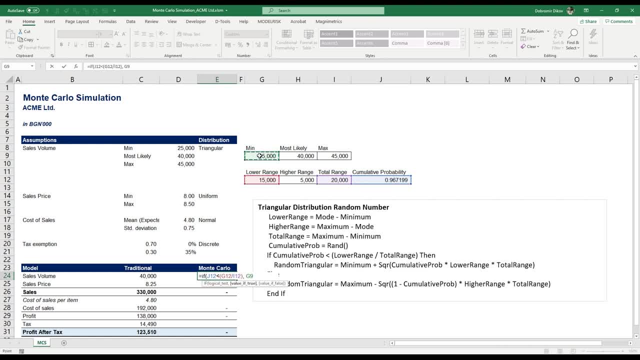 is equal to our minimum Plus the square root of our cumulative probability multiplied by our lower range, multiplied by our total range. And if it's not else, our random triangular is our maximum, So our max Minus the square root of 1 minus our cumulative probability multiplied by the higher range. now, 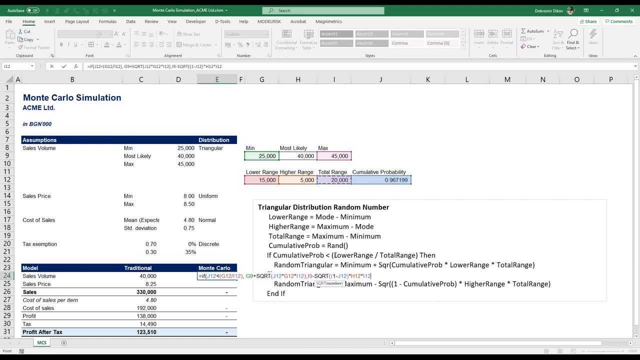 multiplied by the total range: One, two. Okay, that's it, And the easiest way to check if we've written our formula properly is that if our cumulative probability is zero, we need to get 25,, which is the minimum, And if it's one, we need to get 45,, which is the maximum. 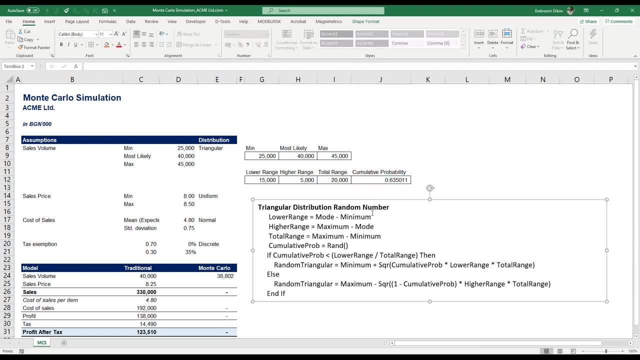 So our formula is correct. Okay, I'm gonna go ahead and get rid of this And let's go ahead and continue with our assumptions below. So for our uniform distribution of sales price, we'll need our min, our max, our max minus min. 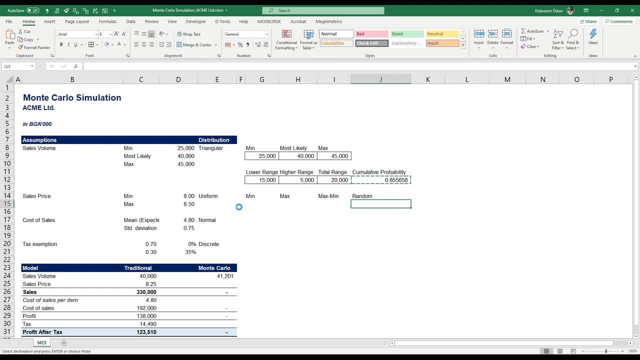 And a random number again. Just gonna copy this random from here And carry over this format. Okay, so our minimum is 8, our maximum is 850. And our max minus our min is 50.. So the way we're going to calculate this is we're going to get the minimum And we're going to add our random between. 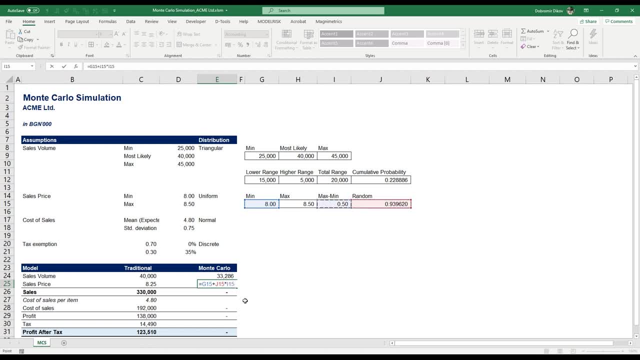 zero and one multiplied by our max minus min. So basically, if our random is zero, we're going to get eight. If our random is one, we're going to get 850.. Okay, now we have our sales, And you see that every time we press F9, our sales change. 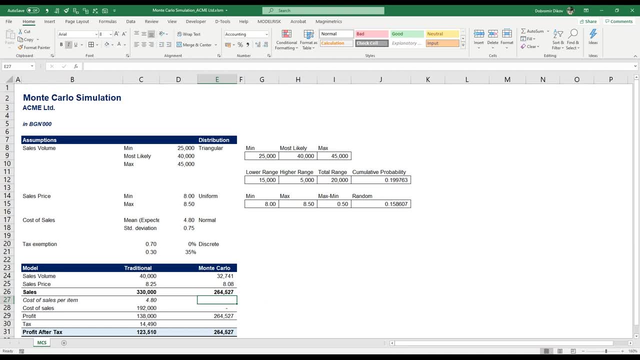 Cost of sales is going to be our normal distribution. So in order to calculate this one, you're gonna have to basically calculate the ratio by itself for sales as well, And in order to get the average, we need our minimum, our stated deviation. 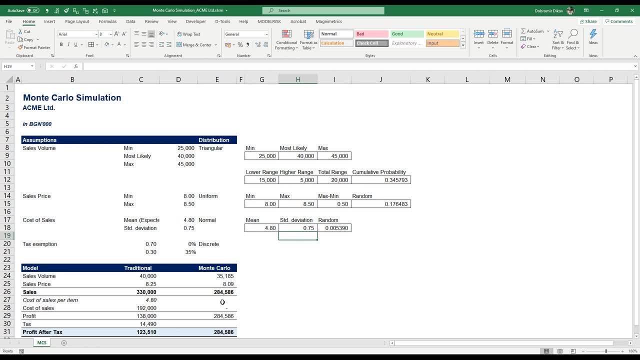 and a random number as well. Okay, so this is our main And this is our standard deviation. Basically it's going to be our min plus norm s inverted, so this returns the inverse of the standard normal cumulative distribution Inverted. this is our probability, so our random multiplied by our standard deviation. 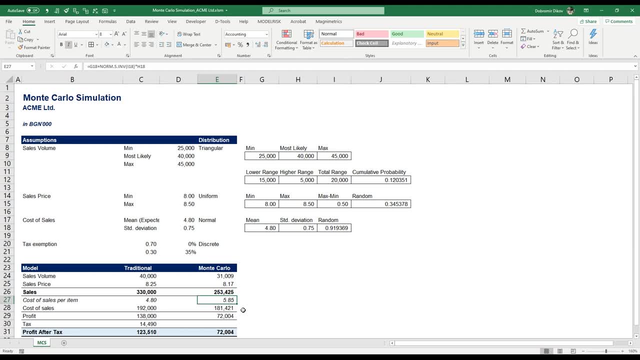 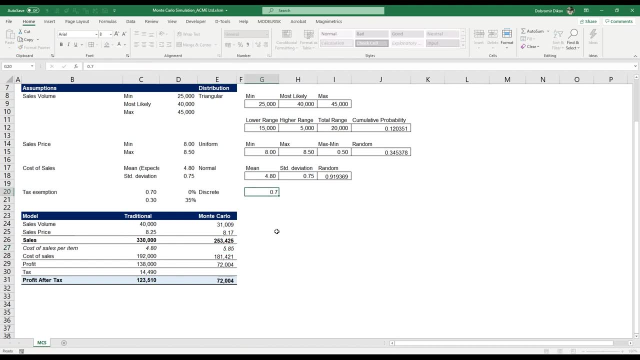 Okay, and what's left here? We have our tax, our discrete, so we have 0.7 chance and 0.3 chance and just grab that random over here. This is at 0.00% And this is at 0.00%. 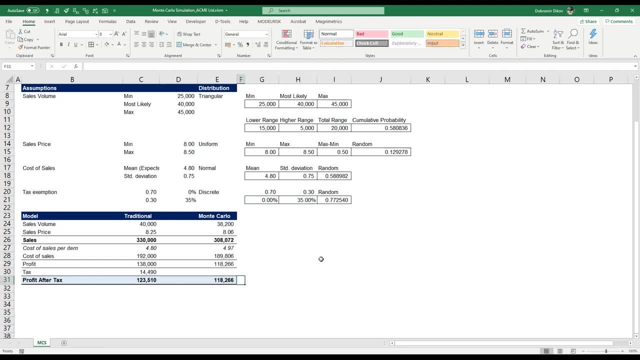 Okay, 35%. The way we're going to calculate that is, we're going to see if our random reaches up to 0.3, it's going to be 35%, and if it continues above that for the next 70%, it's going to. 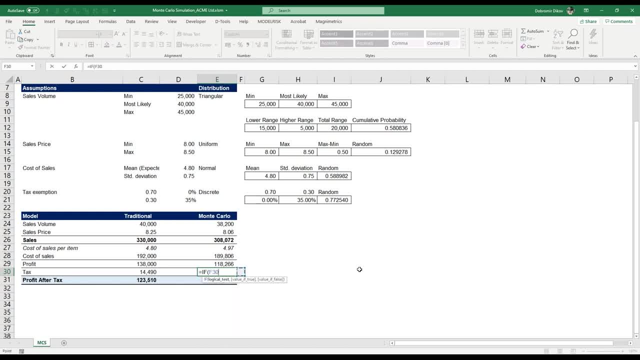 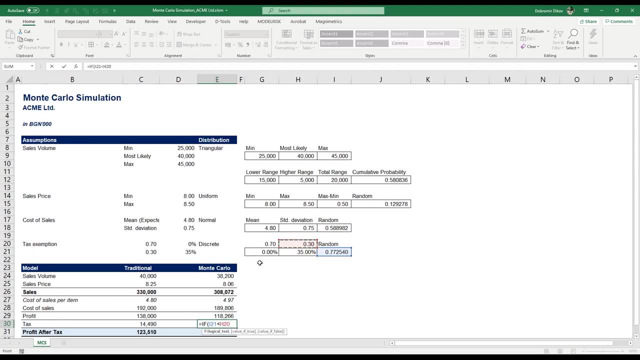 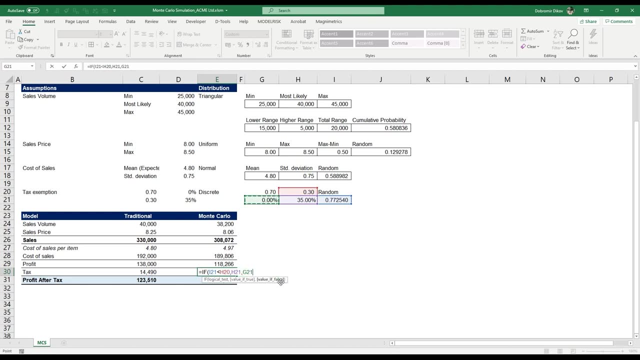 be 0. So if our random is less than this here, give me 35%. Otherwise, give me this 0, multiplied by our profit. Okay, and now you can see that our tax is 0, and if we keep pressing F9, at some point. 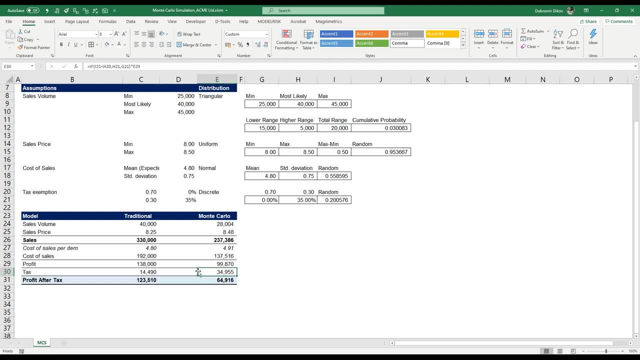 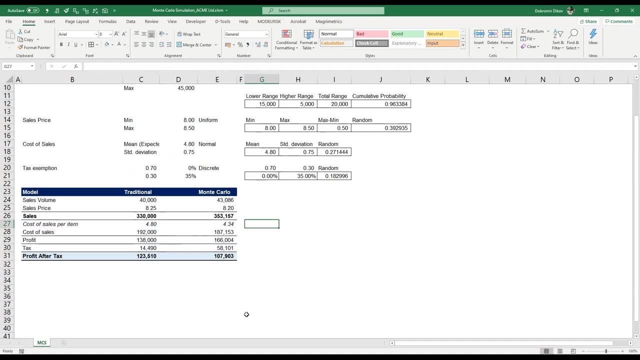 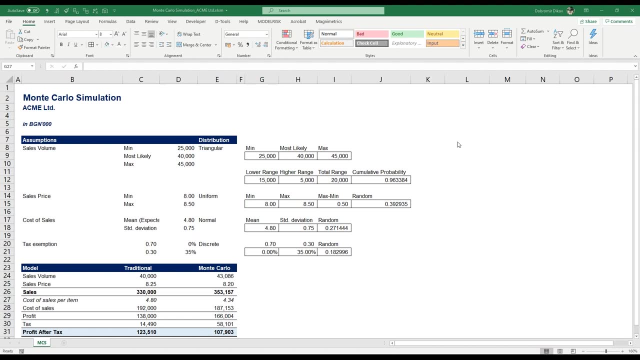 we go into this 0.3 probability and we have a 35% tax. Okay, so that's our Monte Carlo model built here, And now let's see how we can run a simulation. So I'm going to start building it here. 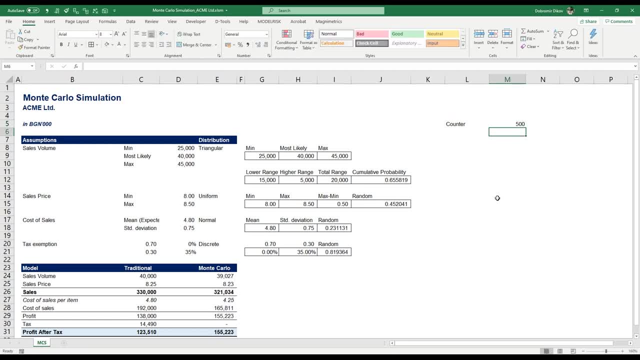 We'll have our counter. This is where we're going to write in how many calculations, how many iterations we want our model to run for. So let's start with 500.. And here we'll have our iterations counter, our average result and our probability of. 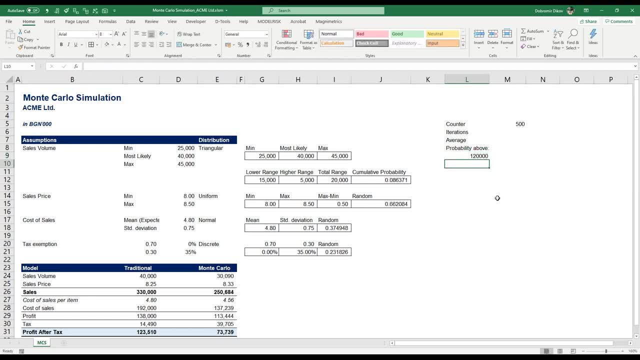 it being above 0.3.. 120,000 and 150,000.. Those are the two checks that we want to do. So if it's above that, we want to consider the project, and if it's above that, we're. 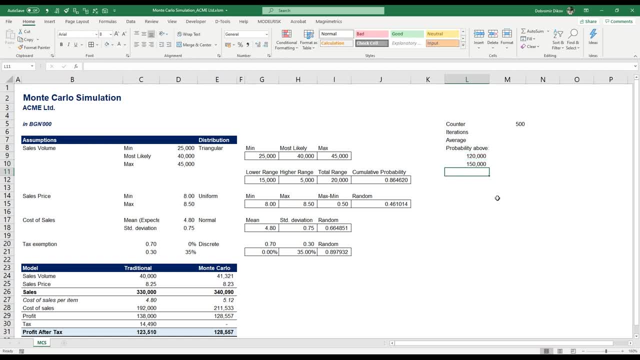 definitely going forward with the project, Okay, and the next thing we need is a list of our iteration and net profit, or profit after tax. I just got net profit that we're going to get. Okay, I'm going to grab that formatting from here. 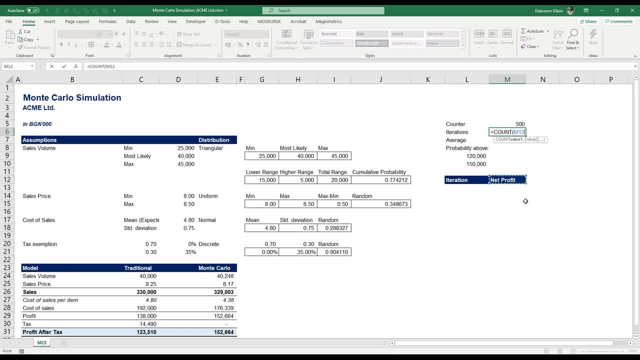 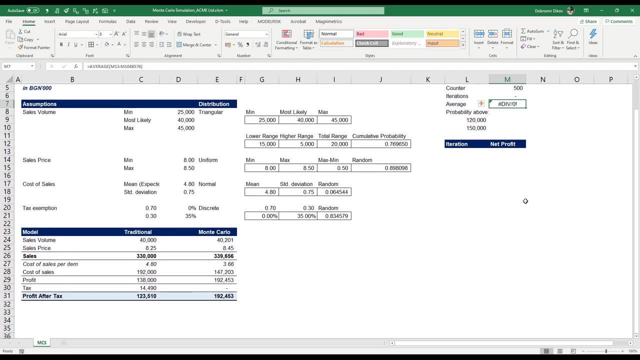 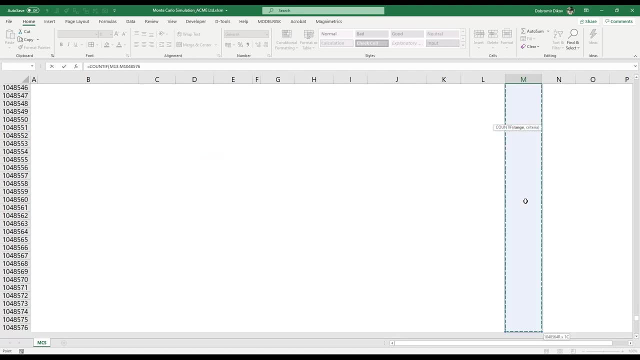 And our iterations is going to be just a count of all our net profits. The average is going to be the same, the average of all those And our probability above. we're going to do it with count if. So, count if, and my just go up here. 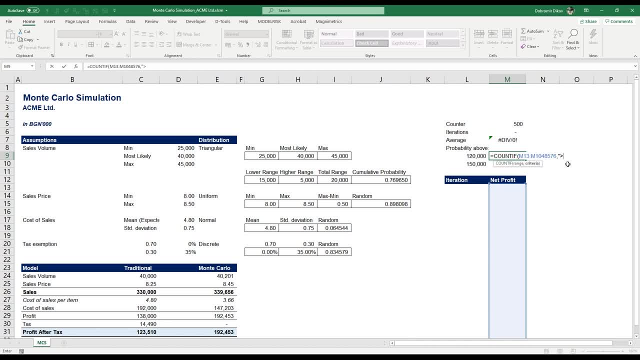 My net profit. Okay, My criteria is going to be above 120,000.. Okay, and I'm going to copy the formula here, paste it here and just switch to 150,000.. Okay, now, how are we going to do that? 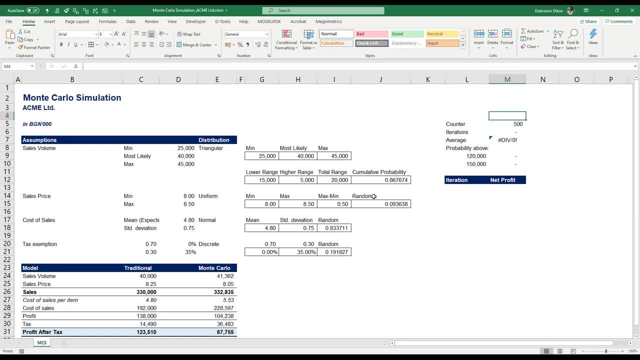 The idea is that we want this to change as if we're pressing F9, and every time it changes, we want this figure to be copied here And going down. One way to do that is by hand, so pressing F9 and copy pasting, but we usually run hundreds. 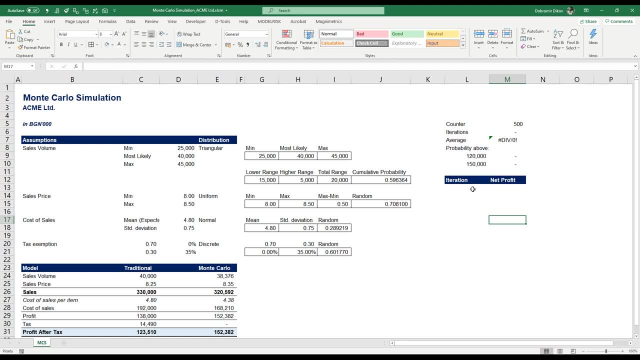 and even thousands of iterations of each simulation, so that's probably not the best idea. What we can do is we can go ahead and write a simple macro to do that for us. Okay, so just going to go to the developer tab insert, going to grab a button, put it. 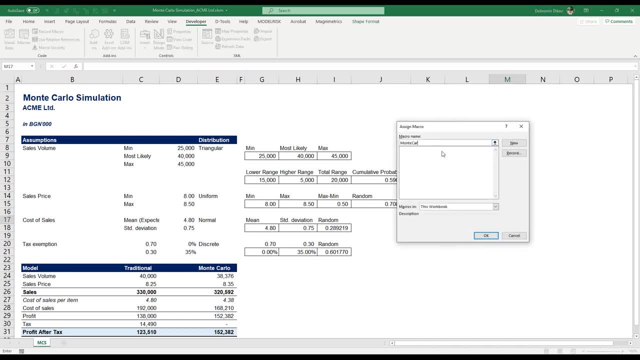 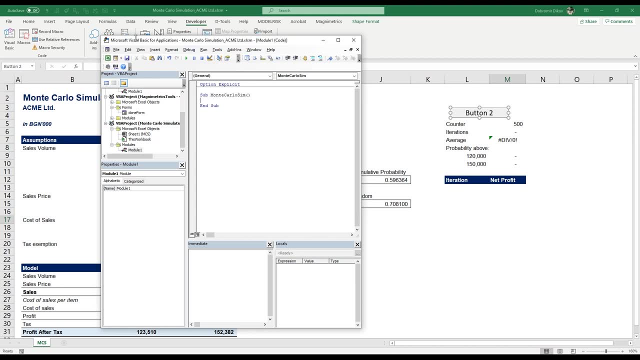 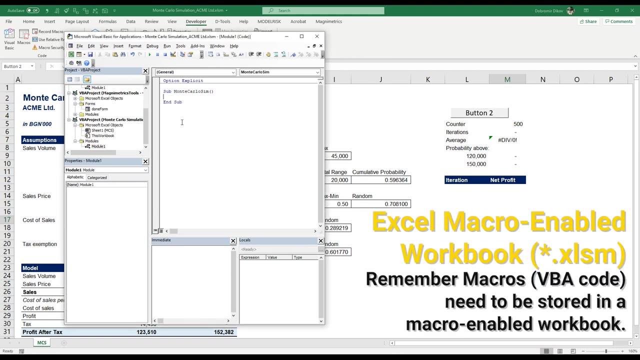 over here and I'm going to call that Monte Carlo Sim and create a new subroutine. So this is our subroutine, This is the Microsoft Visual Basic for Applications editor, and let's just go ahead and write our macro. So what we want is we want a loop that's going to run through our iterations. so for I'm 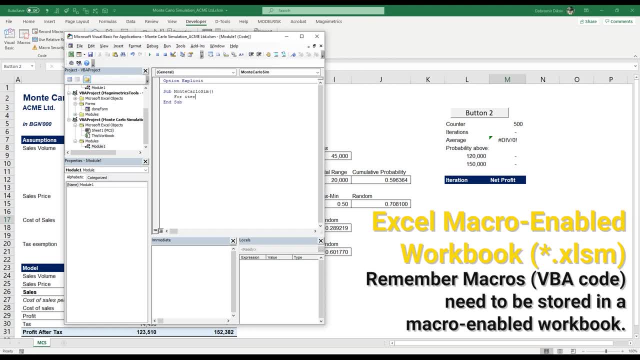 going to call it iterations, Okay, And iteration, and it's going to be from one to cells, row index five. so I want to be getting this here and this is my fifth row and M is my 13th column, so 513, and this: 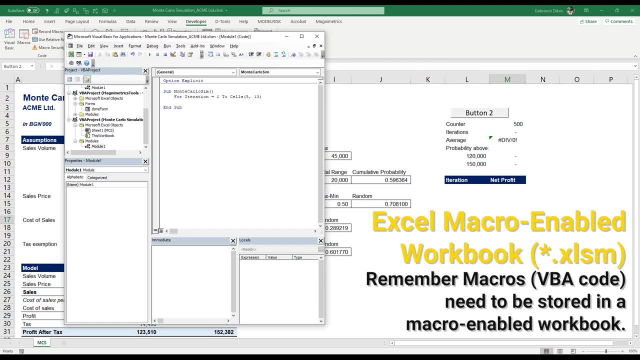 is going to iterate from one to 500, or whatever we type in here, and every four loop needs to end with a next, Okay, Next- iteration. so it's going to go from iteration one, then run everything in between those lines that we're going to input right now and go all the way to 500 before ending. 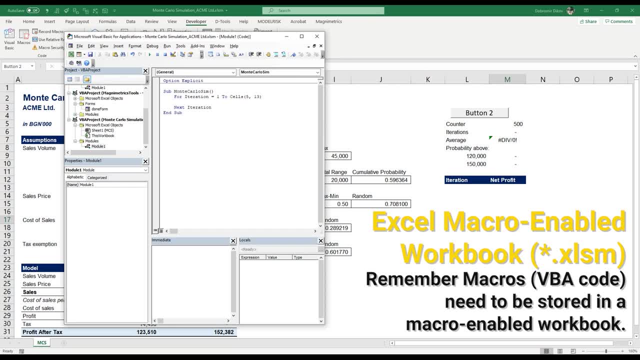 Okay, so what we want it to do, we want our cell. so my iteration heading here is at the 12th row, so I want it to start from the 13th row. So I'm going to type in 12 plus iteration, because our iteration is going to be one. 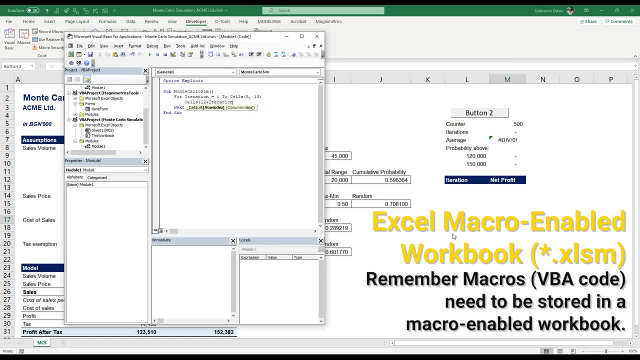 at the first run and then it's going to grow, so it's going to move the cursor down and copy on the next row. every time M is at 13,, and here I wanted to place my result, my net profit, and my net profit is: 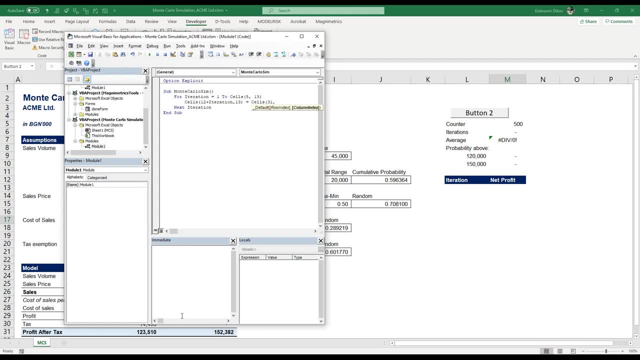 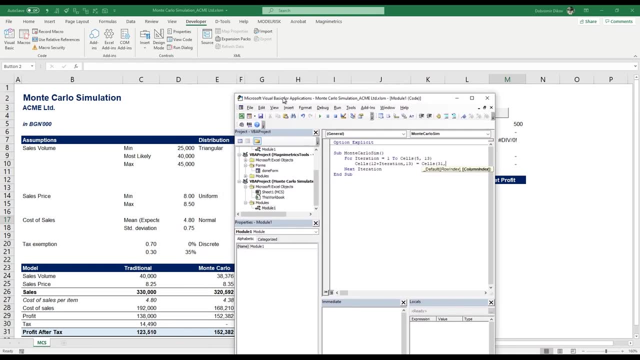 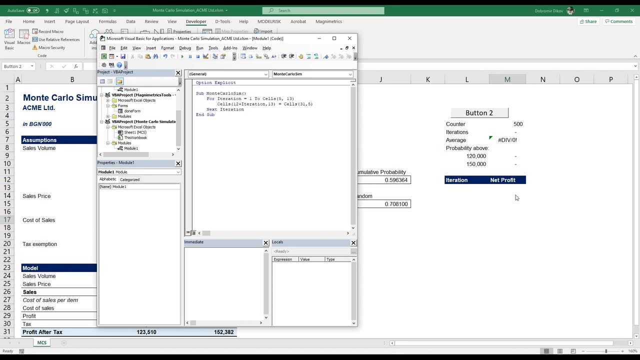 at my 31st row. Okay, Okay. So I'm going to copy this result into my fifth column, so A, B, C, D, E, my fifth column, So 31,, 5.. And every next iteration is going to copy this result in the next row down. 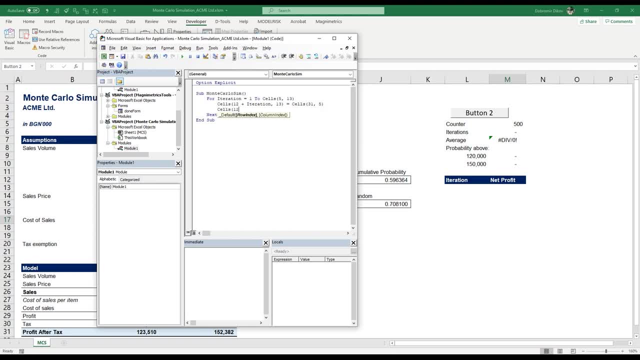 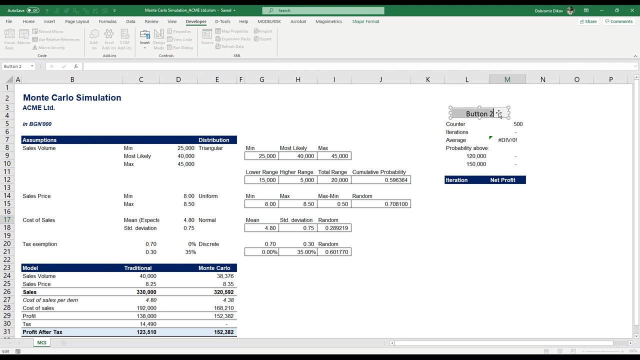 And I also want to have my iteration index. So once again, 12 plus iteration 12, because L is my 12th column, Give me iteration And that's our subroutine, That's our macro. Just save that and just name that a bit more appropriate. 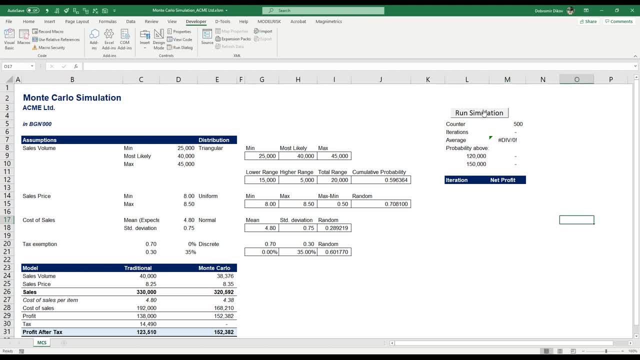 Run simulation. And now the only thing that's left to do is go ahead And run it. Let's first run it for 100 iterations just to see how it works and if it works properly, And let's go ahead run simulation. 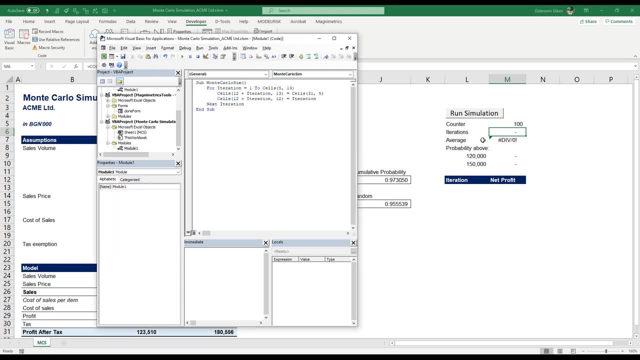 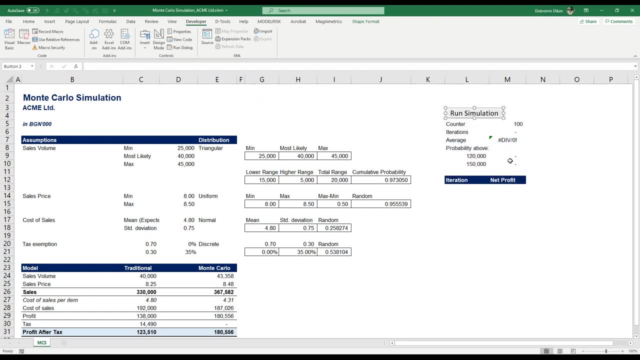 Okay, We have some issue. Okay, Let me just see if we assigned the proper macro, Our term is going to reassign it And now it should work. Yep, Okay, And that's it. We have 100 iterations. We already completed our 100 iterations. 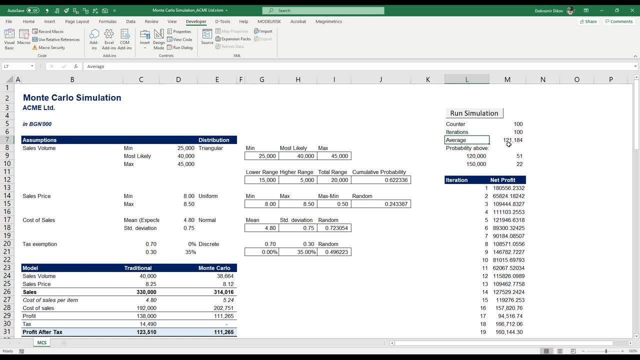 And you can see that the average that we get is 120,000.. And here are all the results from all the iterations. This probability here doesn't seem okay. Yep, We've forgotten something. We just counted the instances And in order to get the probability, we have to divide them over our iterations. 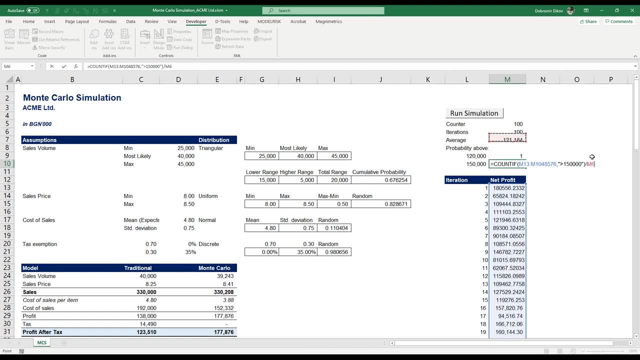 Divide: Okay, And those need to be formatted like: so Okay, I'm going to go ahead and run this for a bit more, just to see if you see that the average now is 121,000. And the probability about it being above 120,000 is about 50%. 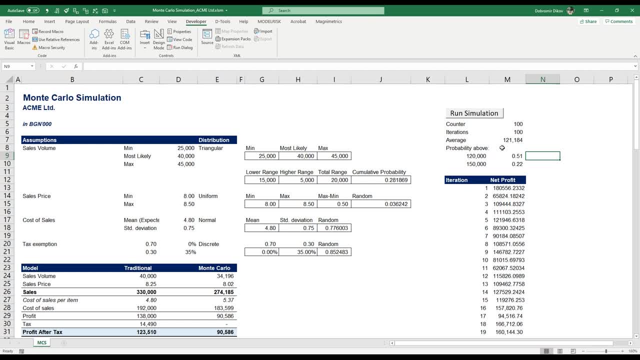 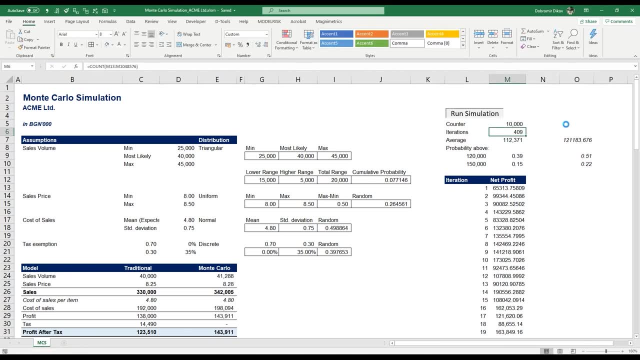 And this is about 22%. But 100 iterations is quite a few, So let's just go ahead and try to run it for about 10,000.. Okay, We've run it for 10,000 iterations And you see that our average dropped a bit. 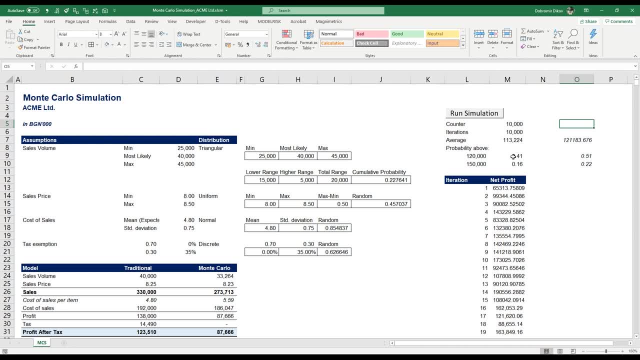 But this is probably enough. iterations: 10,000, if you noticed, like maybe after 5,000, 6,000, it rarely moved from those probabilities And the average pretty much stuck at 113,000.. So we can consider 10,000 iterations enough. 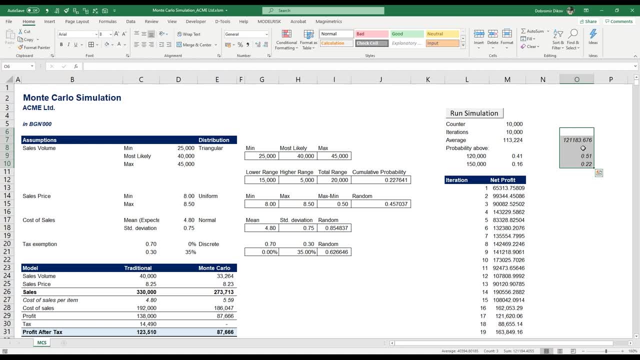 And 100 wasn't enough. It gave us a bit of a misleading information. What we can see here is that the average is 113,000.. That we get, And this means that our probability of it being above 120,000,. what we want is only. 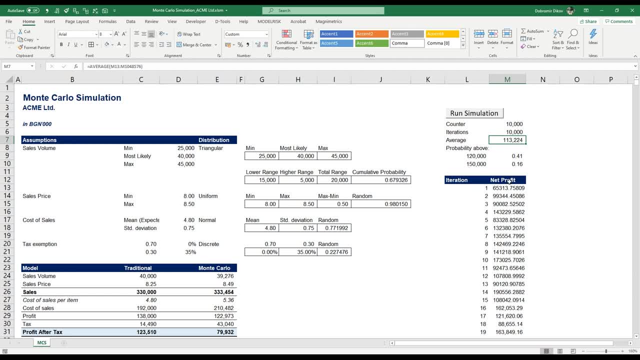 40% and about 150,000,, just about 16%, And you can see that our traditional method here showed us that we're going to get above 120,000, which was a bit misleading, Because once we run our Monte Carlo simulation, you can see that the possibility of that is.